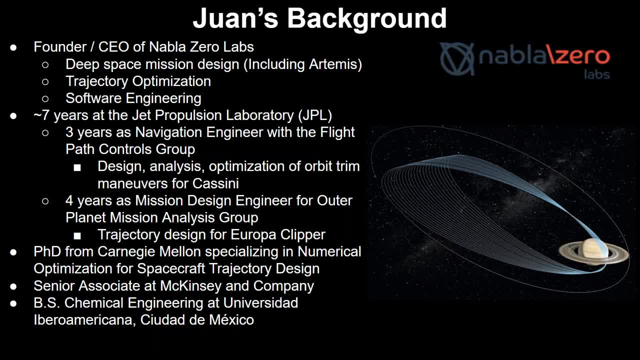 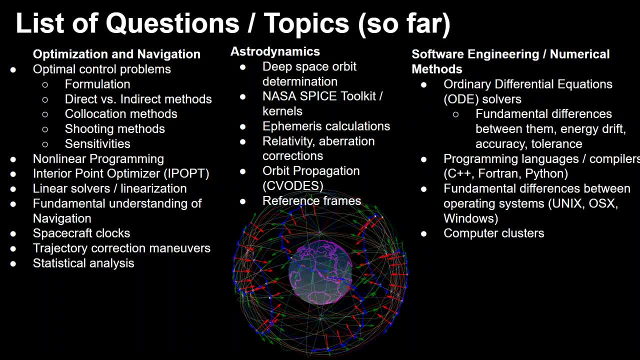 chemical engineering at Universidad Iberoamericana de la Ciudad de Mexico, And some of the questions that I've already have planned out for him, and please let me know in the comments of the YouTube video if you have any other questions that you'd like me to ask him. I'm breaking it down into three. 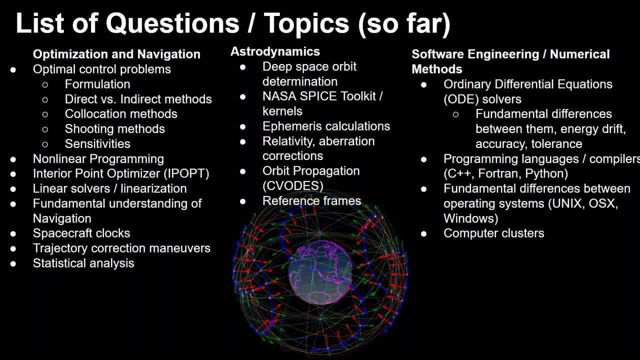 separate topics. So the three separate topics are optimization of navigation, then astrodynamics and then software engineering, slash, numerical methods And realistically they're all going to be related, but I'm going to try to organize it in this way. So for optimization and navigation, 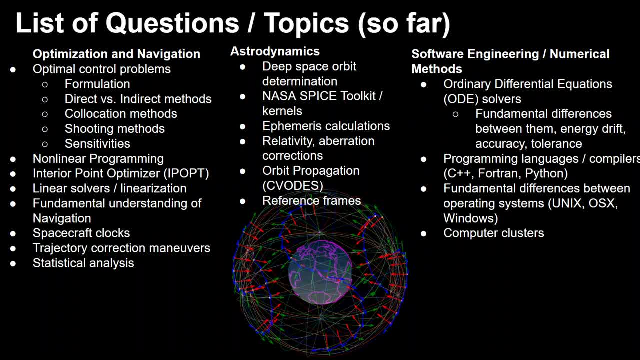 I have optimal control problems, which that has expertise. so how to formulate these problems as far as solving them, direct versus indirect methods, how to use collocation, shooting methods and sensitivities of these solutions? There's nonlinear programming, There's a special or 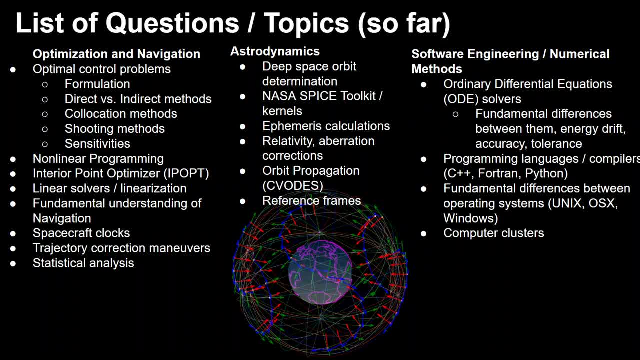 there's one program that he used in his PhD thesis called the Interior Point Optimizer for solving optimal control problems, abbreviated IPOpt. There's linear solvers, slash linearization. in general We're doing this- optimal control problems. And then to navigation. there's a fundamental 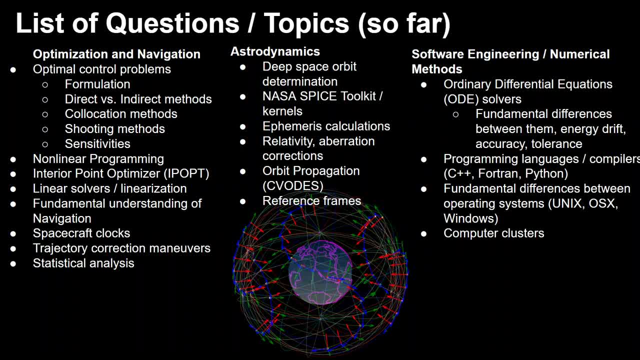 understanding of what navigation is, because there's a general understanding of what GNC guidance, navigation and control is. but actually getting down into the math of what you're actually trying to solve in navigation, I want to learn more about their spacecraft clocks, trajectory correction maneuvers, like he did for Cassini and Europa, and then just statistical analysis involved. 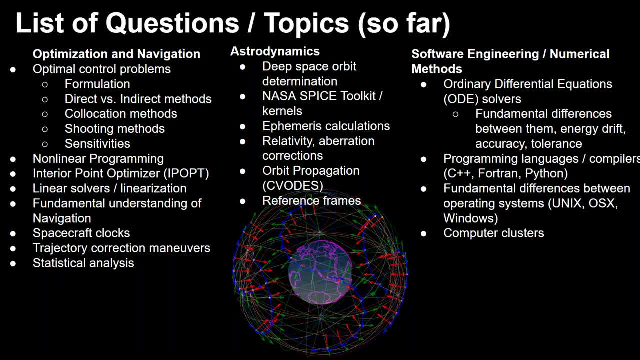 in all this navigation For the astrodynamics. I want to ask him about deep space orbit determination, NASA SPICE toolkit and kernels, which I've shown a lot in the educational videos that I made on the YouTube channel, Ephemeris calculations, which has to do with the SPICE toolkit, Relativity, especially accounting. 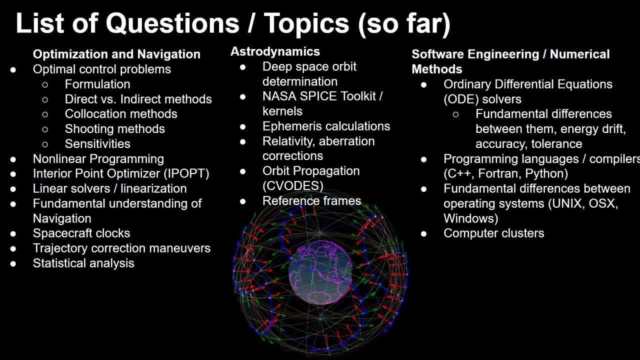 for aberration corrections when getting these ephemeris calculations, Orbit propagation, including different types of solvers and reference frames, And then for the software engineering and numerical methods. I want to get into the fundamentals of ordinary differential equations or ODE solvers, And what are the fundamental differences between the different solvers. 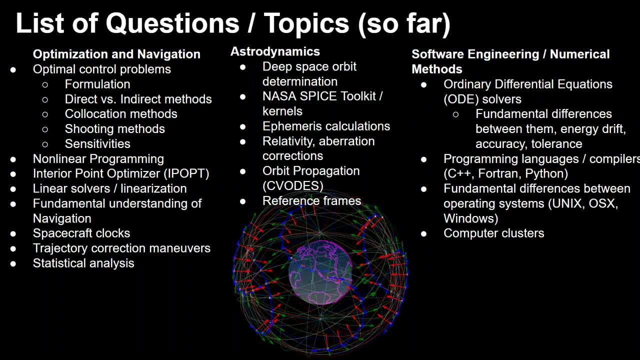 based on, say, energy drift, accuracy and what kind of tolerances you want to use for specific problems. I want to get into that, And then for the astrodynamics, I want to get into the programming languages, slash compilers. So getting into C++, which that is one of his expertises.